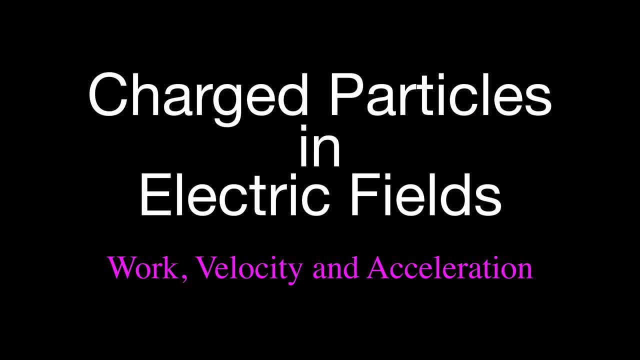 hand corner of this video, we'll go over charged particles that are moving across or perpendicular to the electric field, And in this video we're going to talk about work, velocity and acceleration. Before we get started, please don't forget to subscribe to my channel. 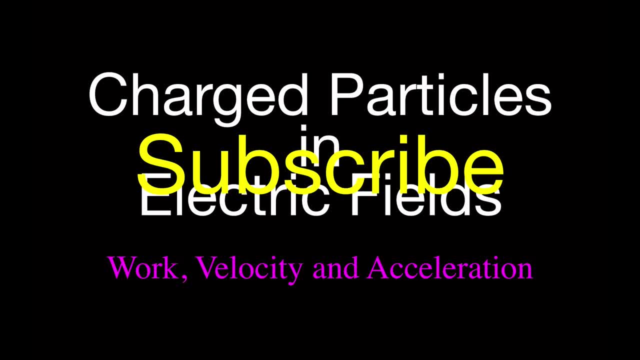 Step-by-Step Science. Please support my channel. Get all my excellent physics, chemistry and math videos. Click on the subscribe button, click on the notification button and get notifications for my channel also. So let's get started. Okay, we're going to. first, we're going to talk about 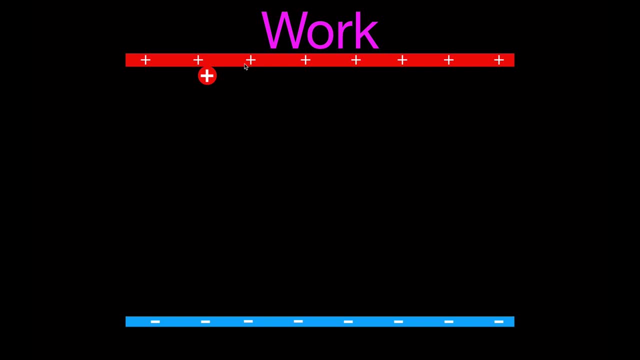 work And what we're going to do is we have this positively charged plate, we have this negatively charged plate and we have this positively charged particle, which is being handled right here because it would be repelled by this positively charged plate, And what we're going to 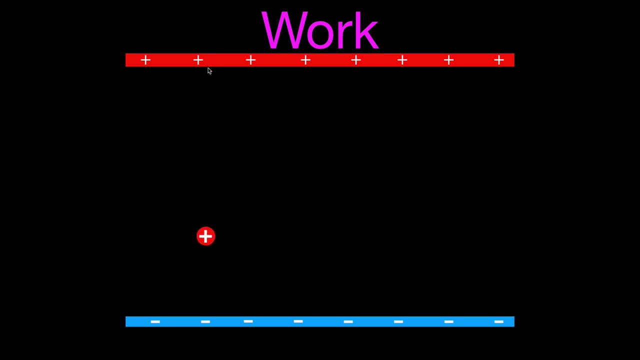 do is we're going to release that particle and it is going to move down towards that negatively charged plate because it will be moving along that electric field. Now we want to talk about is, if I want to move that particle back to the positively charged plate, I would have to apply an external 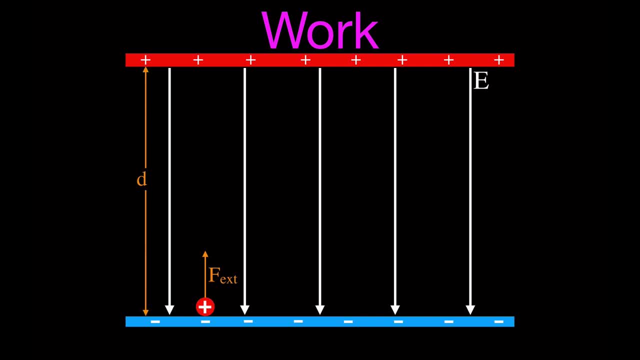 force, I would have to apply that external force over some distance. And when I apply a force over distance or when external force applies a force over distance, then you or that force is doing work. So we move that particle back to the positively charged plate where it doesn't want to. 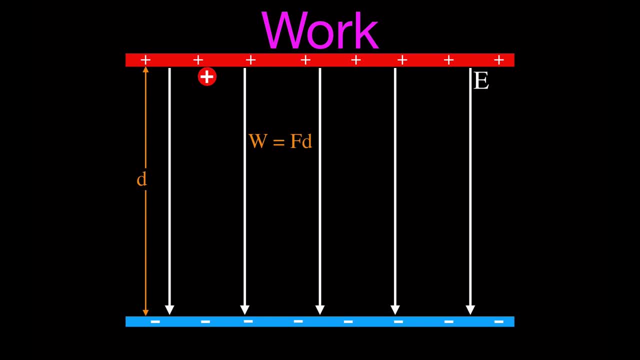 be, then we have to do some work. Now we want to be able to calculate how much work we do and typically, when you get problems like this, you don't get the force times the distance, because that would be too easy. You don't get the force and the distance, because that would be too easy. You get the. 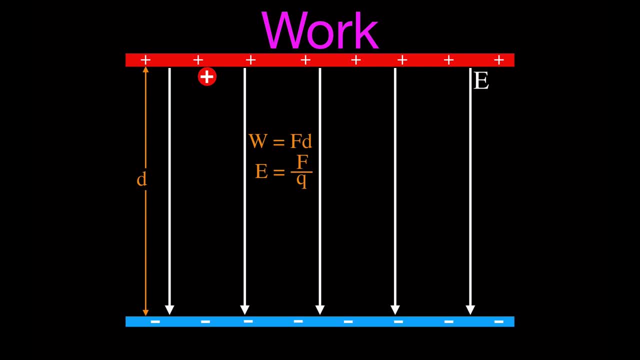 distance, obviously, but then you oftentimes get some information about the electric field, the electric field strength and the charge. So this is the definition of the electric field. The electric field strength is equal to the newtons of force per coulomb of charge. You can see, we have a force. 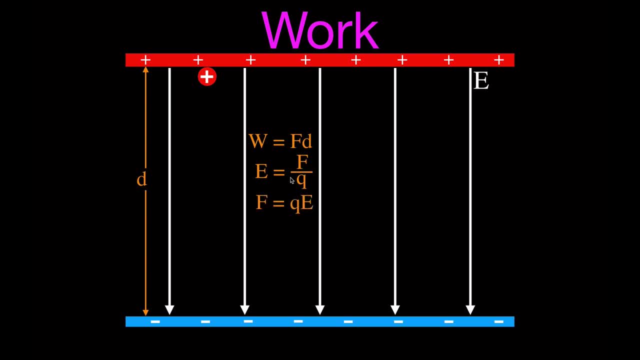 here We have a force. here We're going to solve this equation for the force and then we get: the force is equal to the charge times the electric field strength. I can substitute that value right in here and I get that. the amount of work you do when you. 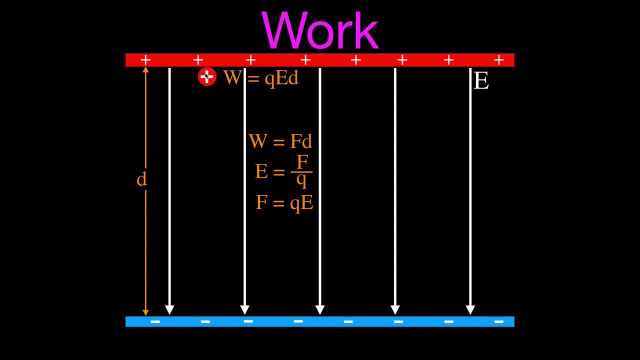 move that charge through that distance. The amount of work you do is equal to the charge in coulombs times the electric field strength times the distance. and don't forget, the distance has to be in meters. Okay, often be given in millimeters or centimeters, All right. so this: 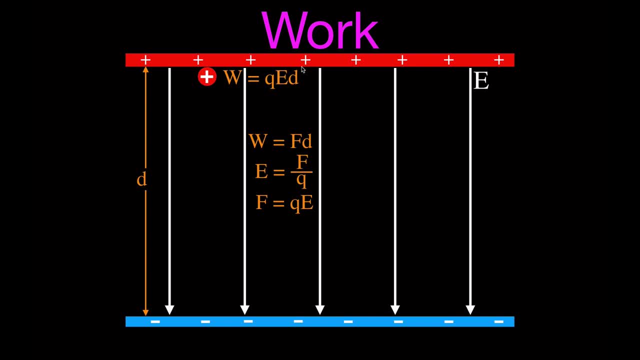 is the equation we can use to calculate the amount of work that the external force does. Now, sometimes you won't be given that information. Maybe you'll be given something about the voltage and the distance or the spawning between the plates. the voltage between the plates. 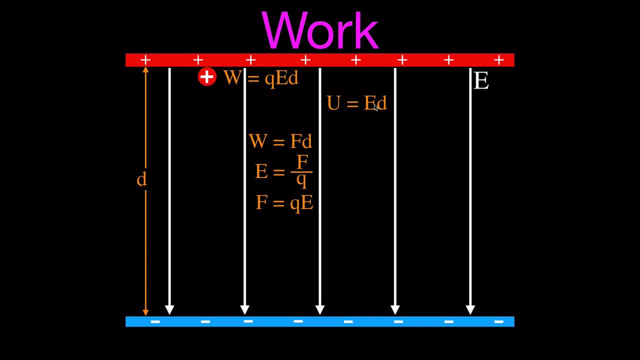 the potential difference. So what I'm going to do is also: you can see, you have here ED and here you have ED. I'm going to substitute this value in here and this is the common equation. You'll see, the amount of work that you do is equal to the charge times the potential difference through which that charge. 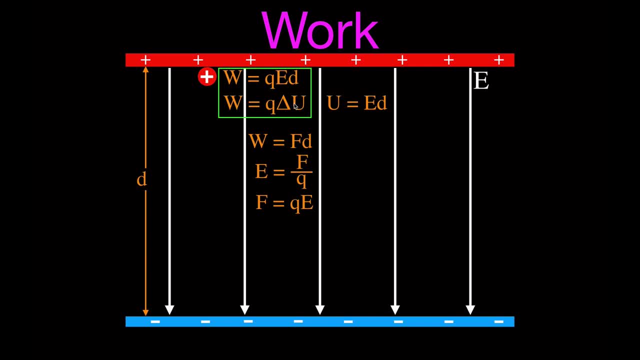 is moved. Okay. so I would say those are the two most common equations you're going to see for calculating the work. I want to point out that if we were to release that particle again, it would fall down, fall back towards that negatively charged plate, because there would be the force. 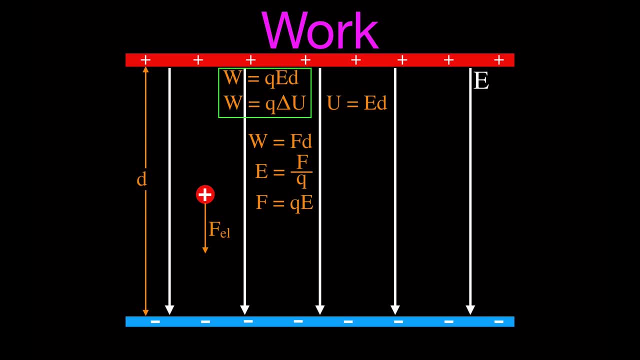 the electric force? Okay, and then the electric force would be applying a force over that distance. that's the same charge. So you could also ask: well, how much work does the electric field do? and it would be equal. Those two values are equal. When we move the charge up, we do some work. The 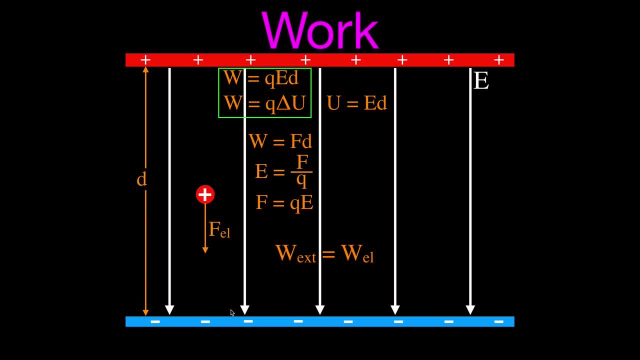 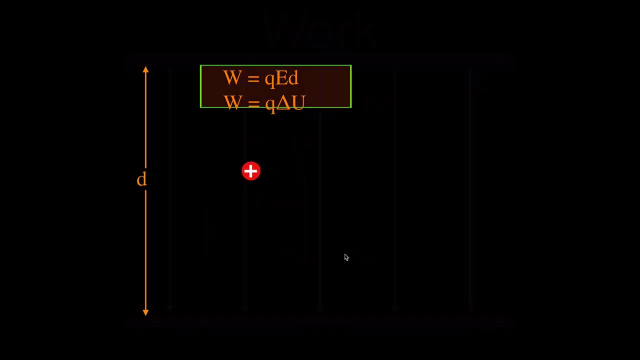 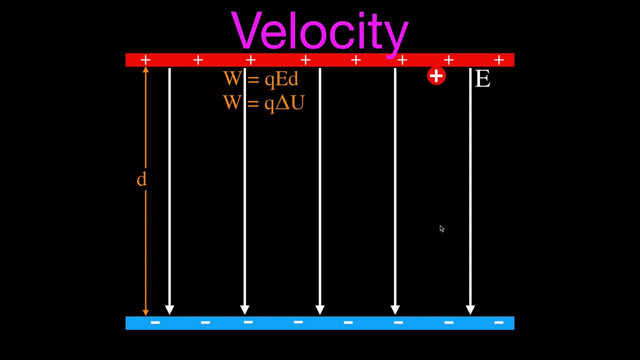 external force does some work and we let it move back to the negative plate, then the work by the electric field, with the electric field is doing that work, and those two values, the magnitude of those two values is the same. Okay, So that's work. Now we can go on and talk about velocity. So we want to figure out now if we have. 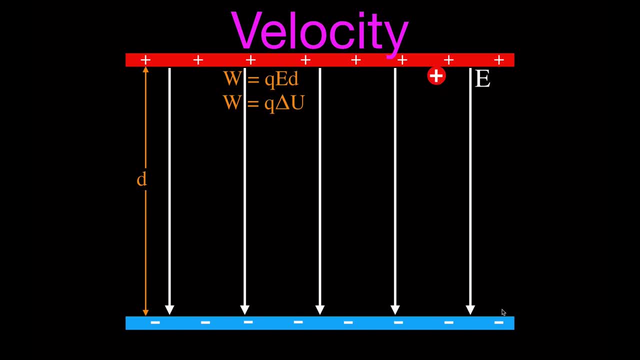 the part of that charge particle right here. we want to know what would its velocity be right before it reaches the negatively charged place. We want to find the velocity here. All right Now. you remember we said that we did some work. This is how we calculate the work When we did work. 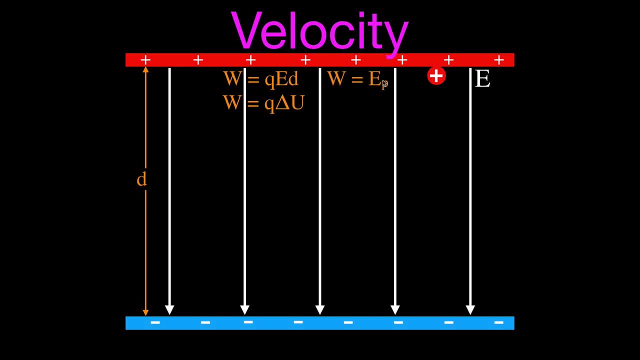 we also gave that charge some electric potential energy Or some potential energy, And it's important to remember that when you raise something up like that through a gravitational field or when you move something like that through an electric field, the amount of work you do is equal to the potential energy Or the potential energy that. 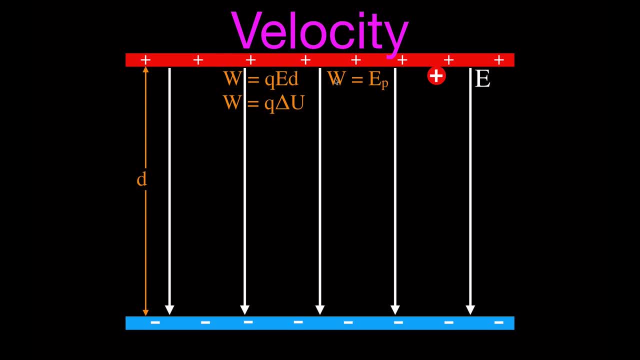 the charge would have would be equal to the amount of work that you did. Okay, Now what happens when we release the particle? we've seen it falls or moves back towards the negative plate. That means it's losing potential energy As the distance between the charge and the negative plate. 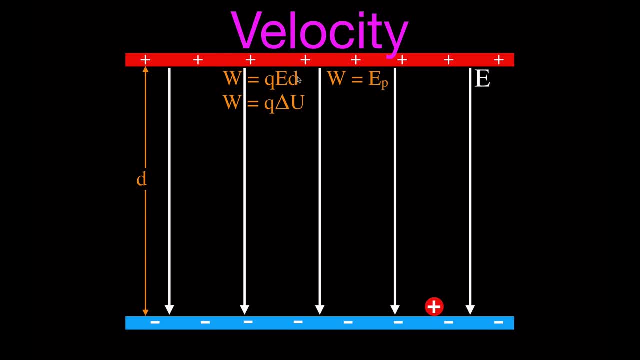 decreases, then it's going to have a lot of energy. So we're going to have a lot of energy. We're going to have less potential energy because the distance is going to be less. Well, where did that potential energy go? That potential energy went into the motion of the particle as it speeds. 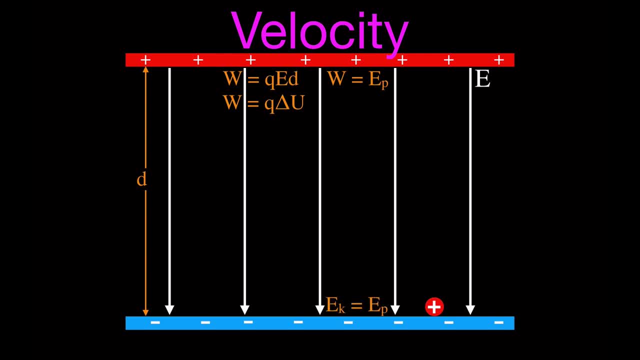 up as it increases its velocity, So it's going to convert it into kinetic energy. So we have work, We have potential energy And we let the particle move back to the negative plate and then it has kinetic energy. So at the bottom here, at the negative plate, the amount of potential energy. 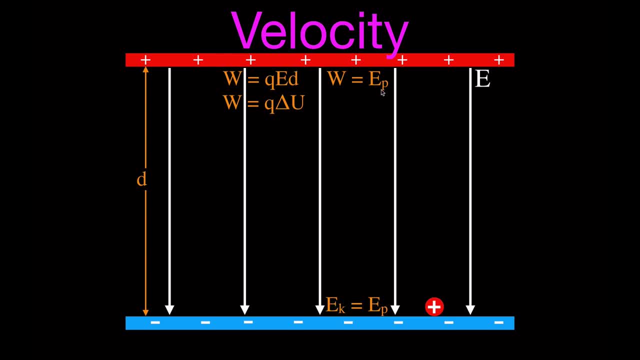 is equal- to excuse me- The amount of kinetic energy is going to be equal to the amount of potential energy it had here. So I just want to point out really quickly, please remember, that the amount of work you do is equal to the potential energy. you give the particle And then we let the particle move. The amount of 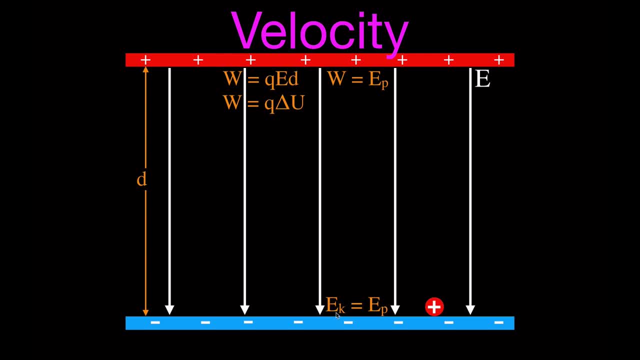 potential energy is going to be equal to the kinetic energy here at the bottom. Here it has potential and no kinetic. Here it has kinetic but no potential, because the distance basically between the particle and the plate is zero. Now we can use this relationship, this conservation. 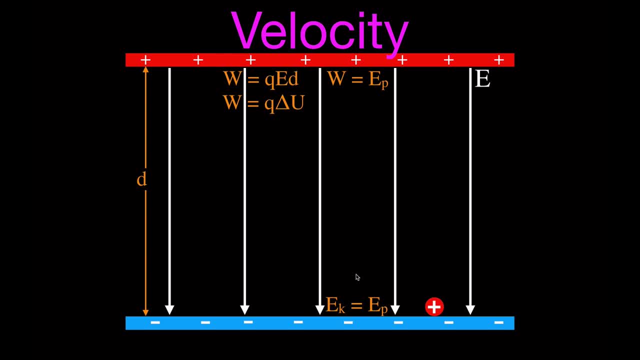 of energy relationship to calculate the velocity, Because we know that the kinetic energy is one half mv squared. That's the same equation we use for mechanics And we figured out here that the potential energy is equal to qed. I want to just take this equation and solve it for velocity. 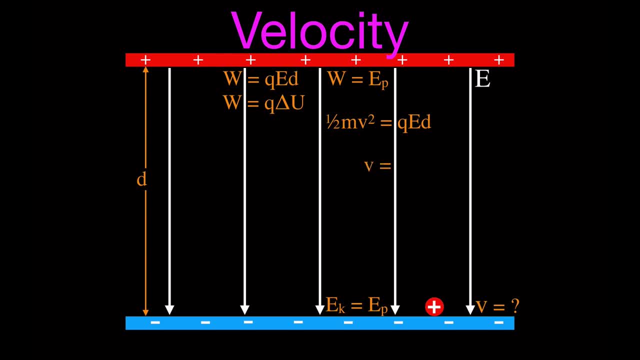 Okay, in order to do that, I have to do a couple steps, But let me just show you the equation we get and then I'll show you or go over the steps. The velocity is going to be equal to the square root of two times q, times e, times d, divided by the mass of that particle. Now, how did I do? 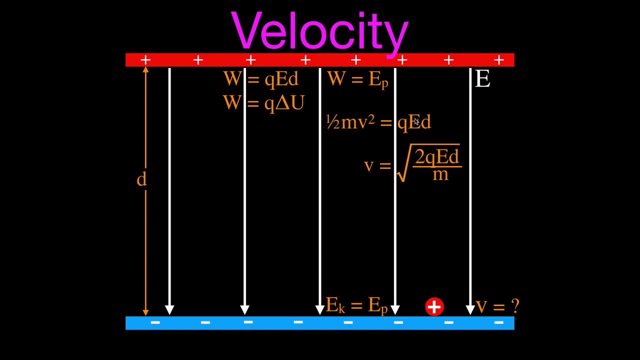 that You can see, I have to convert or have to move all this other stuff to the other side- The half, the m and the squared. So what I'm going to do first, what I did first, was I multiplied by two and you get two qed. that gets rid of the half. Divide by m, you divide by m and then you take the. 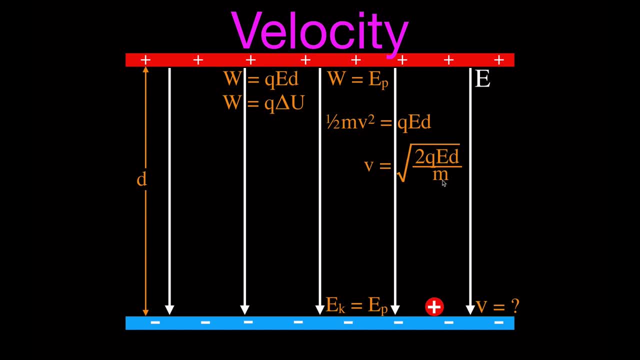 square root and you get that the velocity is equal to the square root of two qed divided by m. Now remember that We can also say: the work is q through the, through the potential width that it's moved. So I can actually substitute that value in and then we can get two different equations. These equations are: 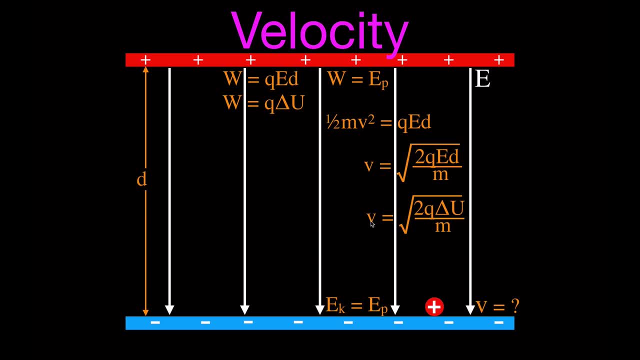 the same equation for the velocity just depends what information are you given. Okay, so we have two equations and we can use those two, those two equations, to calculate the velocity at the bottom, here, or really any place, depending on the distance or the spinal through which it's moved. Okay, we. 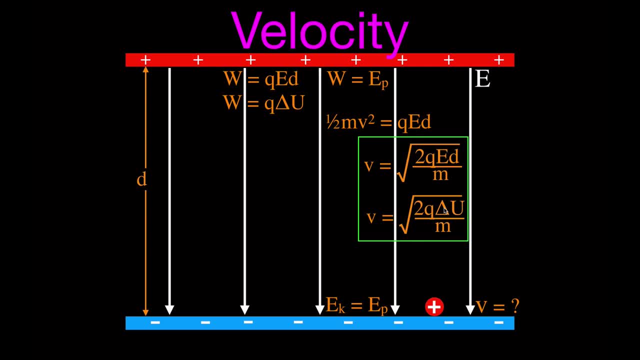 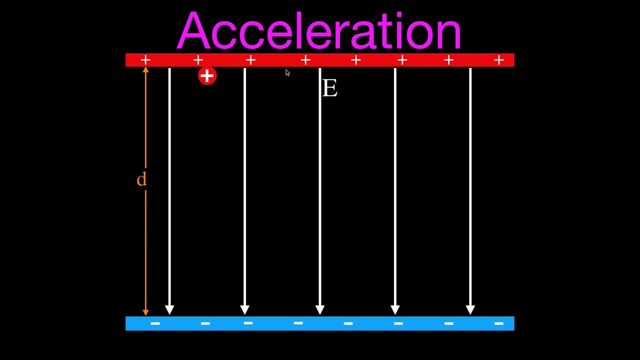 did work, and now we did velocity, And now we're going to talk about the acceleration. Okay, the acceleration it's moving through a homogenous electric field. Don't forget: the electric field goes from the positive plate to the negative plate and it's going to be moving through that homogenous electric field. So it's. 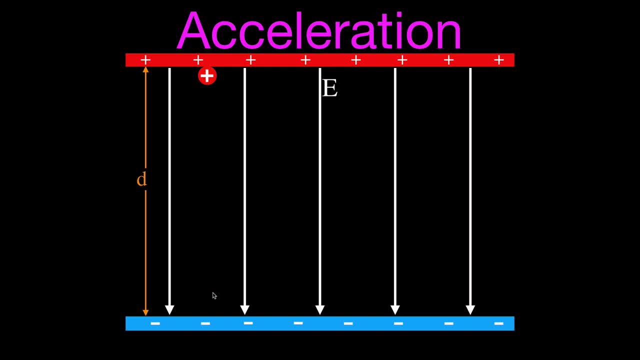 going to have a constant velocity- excuse me, not constant velocity- an increasing velocity and a constant acceleration. The acceleration we can calculate using Newton's second law, because we know there'll be some force, It has some mass, that particle, and we can calculate the velocity. 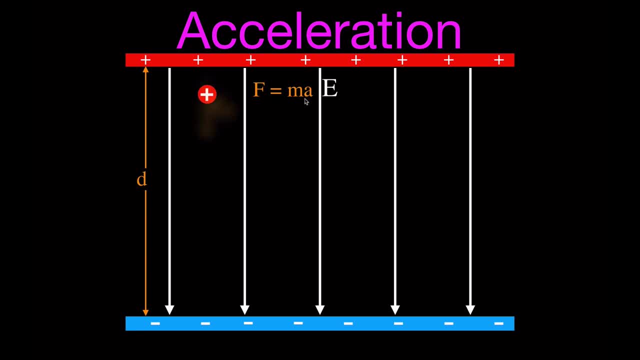 We can calculate the acceleration using: f equals ma. We can rearrange that equation. when that falls down, it's going to be accelerating. We get that the acceleration is equal to the force divided by the mass. Now the force this time is the force from the electric field, which we can calculate using: 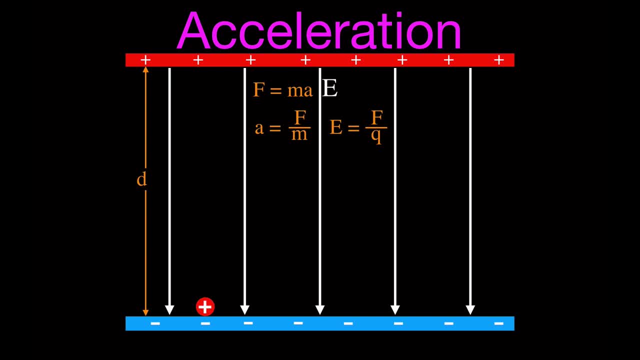 the same equation that the electric field strength is equal to the newtons of force divided by or per coulomb of charge. Rearrange and solve for the force. again We get qe, and then I can substitute that into my acceleration. So I can calculate the acceleration using. f equals ma. We can rearrange. 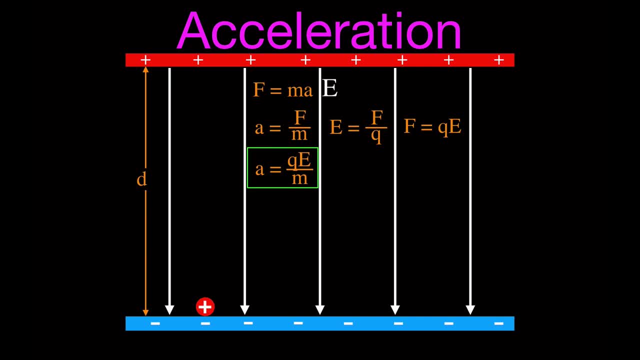 the acceleration equation, and I get that. the acceleration is equal to the coulombs of charge times, the electric field strength divided by the mass of the particle. Okay, so that's one equation. Now, remember we also said we have that the potential between the plates is equal to the 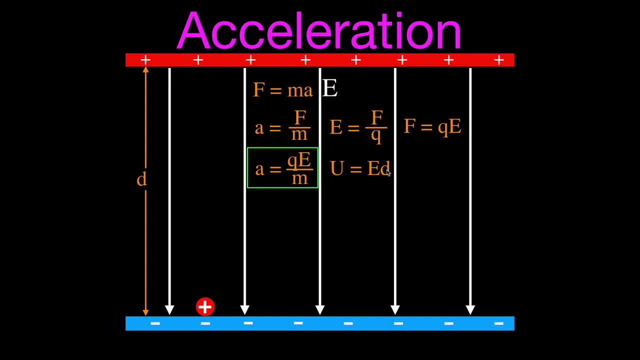 electric field strength times the distance. So I can come up with my second equation by solving this equation for the electric field strength and substituting the electric field strength for the mass of the particle. So I can come up with my second equation by substituting that in here and then I get that the 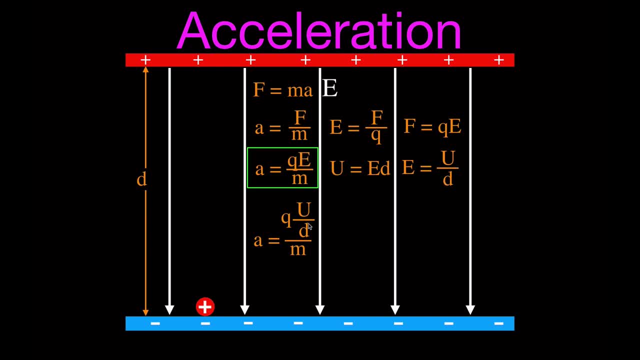 acceleration is equal to q. This is this: q E, remember now, is equal to ud divided by m. Now I can clean this up a little bit and I can get that the acceleration is equal to q. the coulombs of charge times the potential difference to which it's moved, then the mass of the particle and the actual 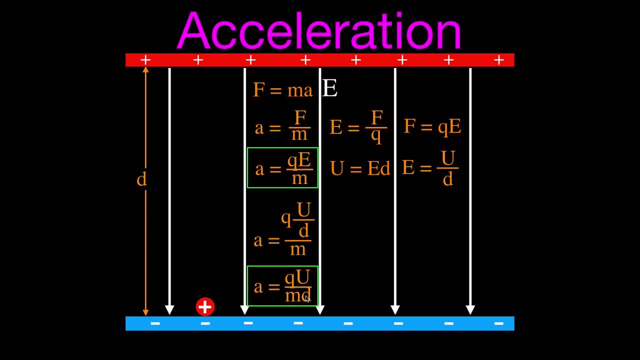 distance, the physical distance between those two plates. So once again we have two equations for the acceleration. We had two for work, two for velocity and two for the acceleration, depending what information you're given. Now here we have all six equations. I just put them on the summary. 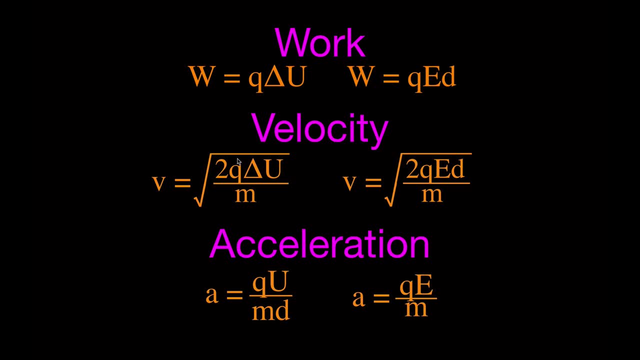 page. Basically, this equation and this equation are the same, this and this and this. Once again, it depends on which information are you given. For example, here you're given the charge and the charge, but are you given the potential difference And here you're given the electric? 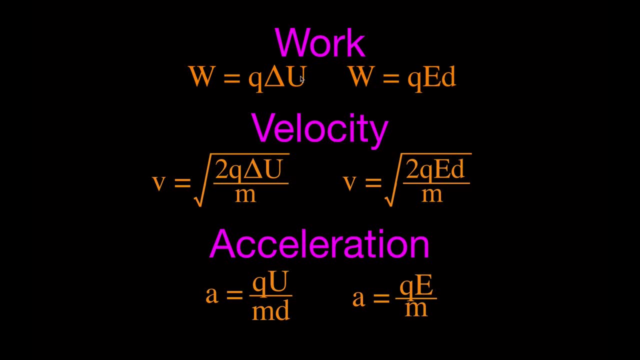 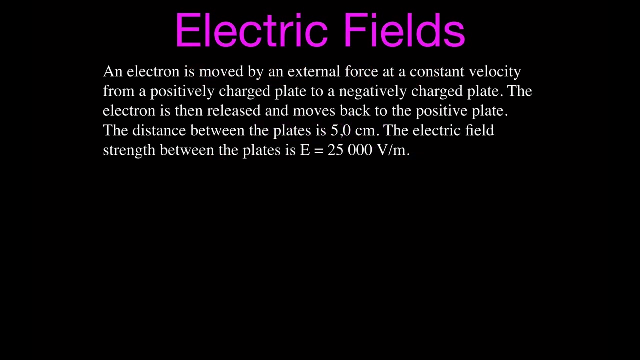 field strength and the distance, because u is equal to e times d. Okay, So that is how we can calculate the work, the velocity and the acceleration. So this is the example problem that we're going to go through for this video. It says: here we have an electron, so it's negatively. 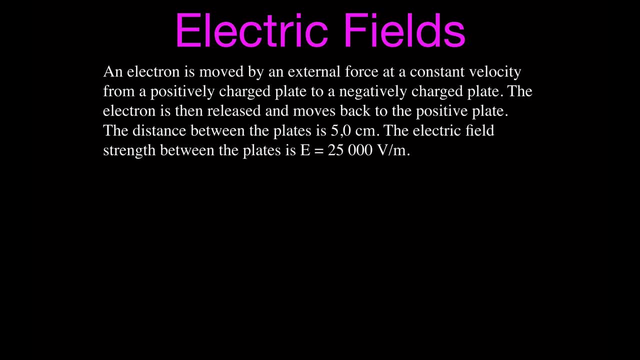 charged. It moves by an external force at a constant velocity from a positively charged plate to a negatively charged plate. The electron is then released and it moves back to the positive plate. The distance between the plates is five centimeters and the electric field strength. 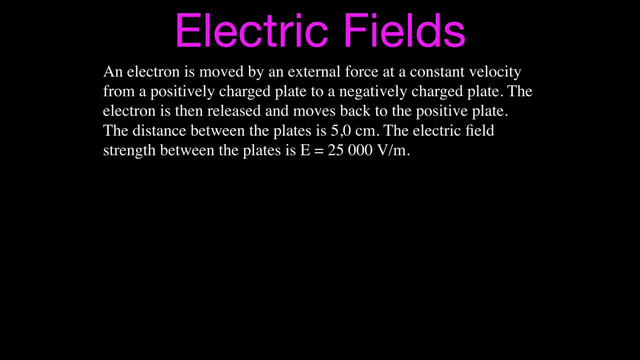 between the plates is 25 volts per meter. Okay, and we're going to answer the following four questions. I think you have four questions here. How much work must be done by the external force to move that electron to the positive plate? or, excuse me, from the positive to the negative We want. 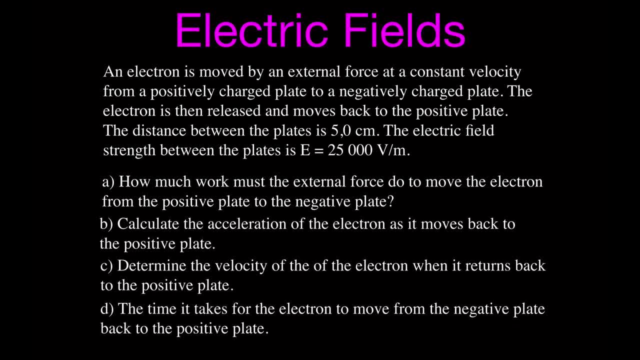 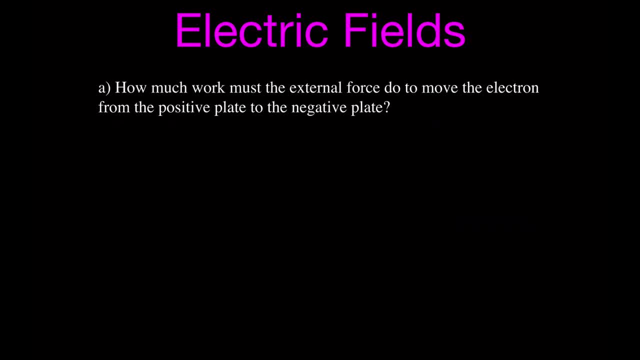 to calculate the acceleration, we want to calculate the velocity and we want to calculate the time it takes for the electron to move when we release it from the negative plate back to the positive plate. So we're going to do these each one at a time. It's just what we went through in the 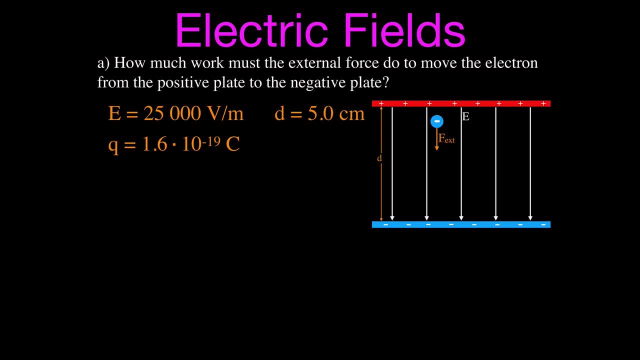 previous examples. The explanation that we went over it says here how much work must be done by the external force to move the electron from the positive plate to the negative plate. Okay, So you can see. here's our electron, here's our positive plate. 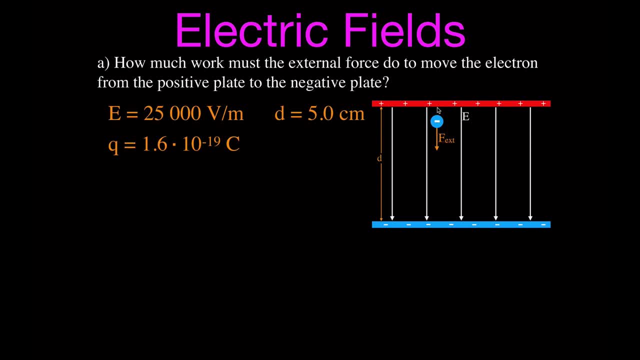 It would normally want to be stuck on that positive plate, because they're attracting, because they have opposite charges. In order to move it away and to move it here, we're going to have to apply a force over distance. That's why we have this external force. 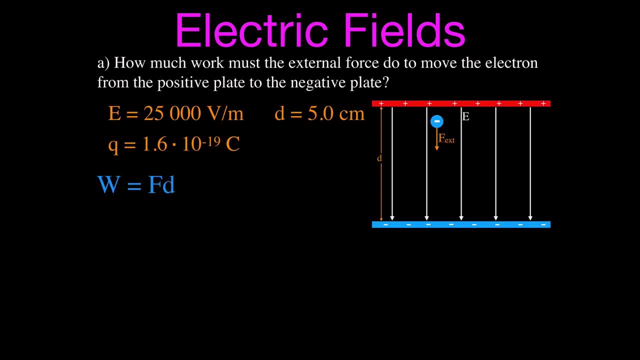 And you'll remember, the amount of work is equal to the force times the distance. We have our electric field definition. We solve that for F and we get QE and we get that the work is equal to QED- the charge, the electric field strength and the distance. 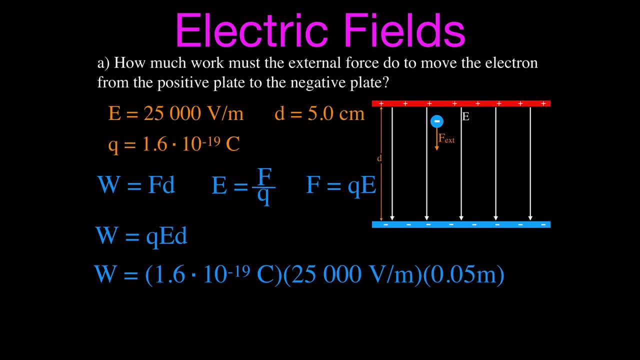 And that is what we were given, And therefore we can just say that the amount of work is equal to the charge on electron 1.6 times 10. to the minus 19 coulomb, This is 25,000 volts per meter. 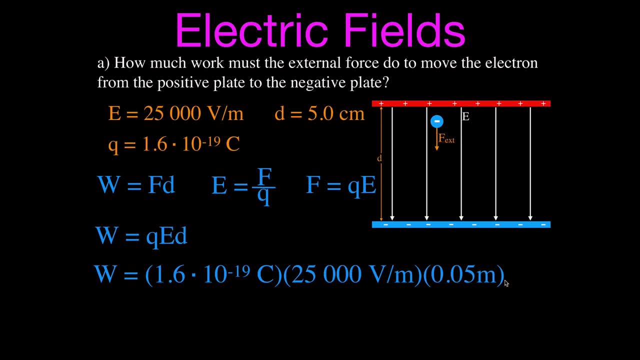 That's the electric field strength And this is the distance in meters. Don't forget. you're given centimeters, You have to convert to meters And you get that the amount of work that you would do in moving that electron would be 2.0 times 10 to the minus 16.. 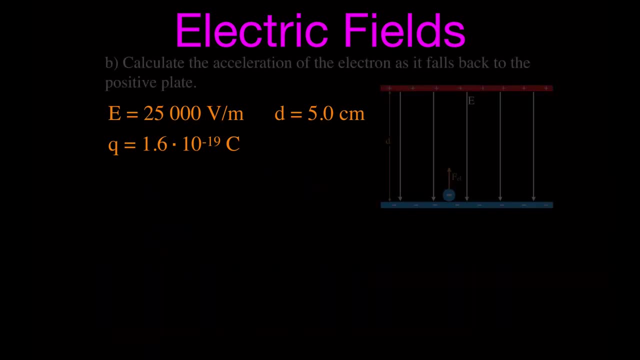 Joules. OK, Letter B Now it says: calculate the acceleration. Now we have the electron here at the negative plate. They're going to repel each other. So it's going to be accelerated through that homogenous electric field And we know that the force is equal to the mass times. acceleration for Newton's second. 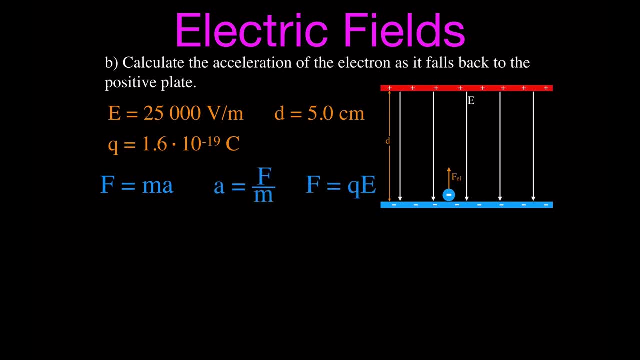 law The acceleration is the force divided by the mass. And we have our kind of our definition for the electric field strength solved for F the force, And we can substitute that in and we get the acceleration is equal to The charge divided by the electric field strength divided by the mass of the electron. 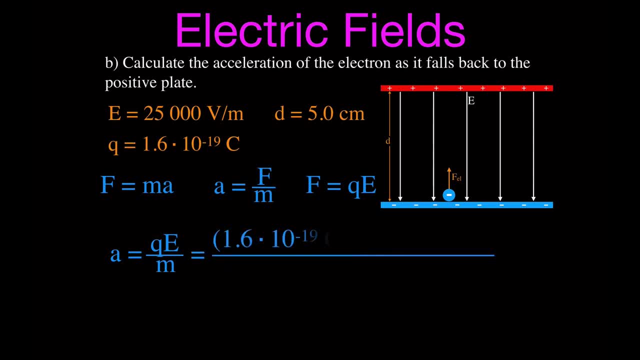 which will give you, of course, but you could just look it up- And Q, the charge is the same and the electric field strength is the same, And this time the mass of the electron, or the mass electron, is always 9.1 times 10 to. 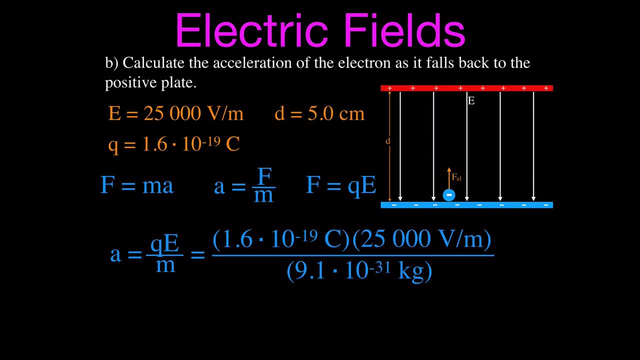 the minus 31 kilograms. And if you do all of that then you get an acceleration of 4.4 times 10 to the 15 meters per second, squared, OK. Constant acceleration through that homogenous electric field, OK. And now we want to know the velocity. 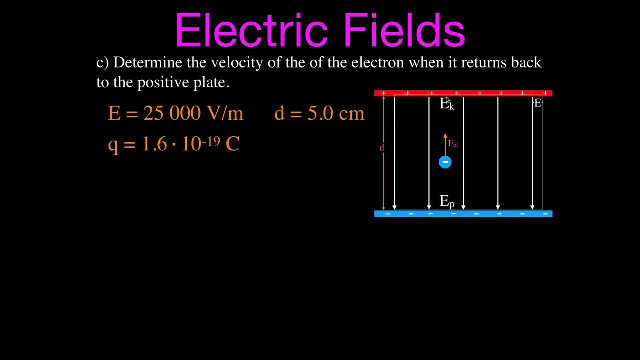 Now it's moving back from the force, from the electric field, And we want to know what the velocity is when it gets right here. Don't forget that we said we have potential energy when we move that charge through that field. We did work. 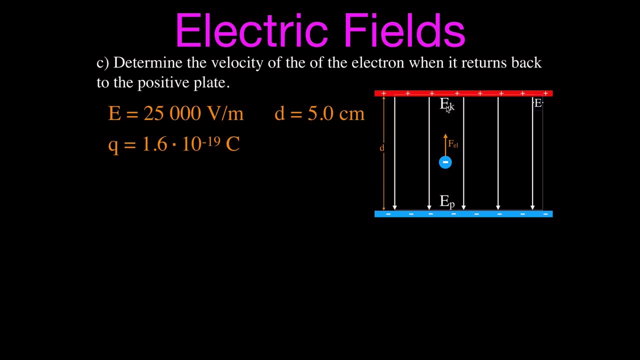 We gave it potential energy And that's going to be equal to the kinetic energy when right there at that positive plate. So we can set those two values equal to each other. Conservation of energy: 1 half mv squared equals Qed. Solve for the velocity, as I showed you previously. 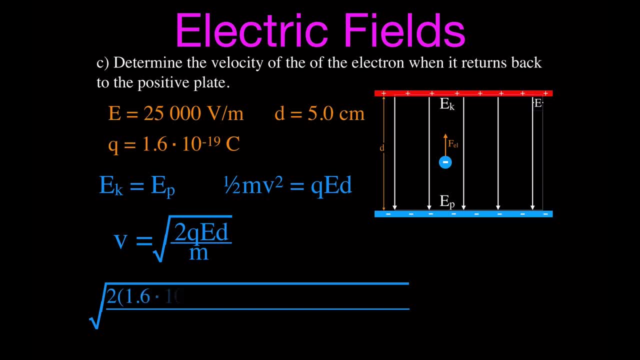 And we can just plug those values in 2 times Q. Q is the charge, volts per meter is the electric field, strength the distance, And this time we're going to divide by the mass. Do all that, take the square root and you get that. 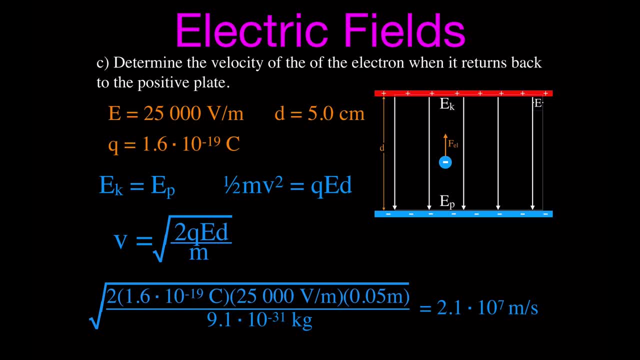 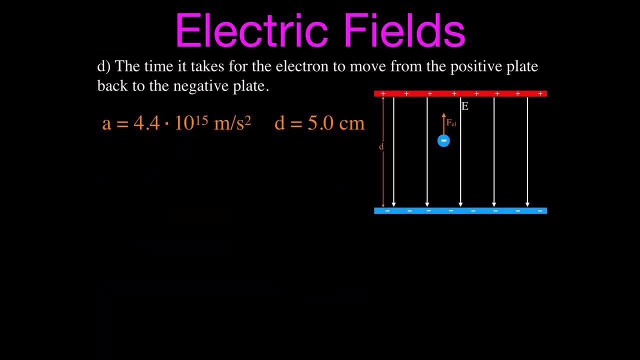 That is 2.1 times 10 to the 7 meters per second squared OK. Letter D. the last thing It says here: the time it takes for the electron to move from the positive plate back to the negative plate. OK. 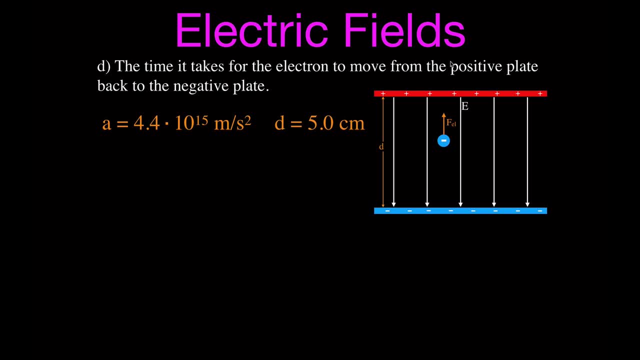 We want to move it from the positive plate back to the negative plate. This should obviously say from the negative plate back to the positive plate. So that's the direction it's going to be moving, And so I have this positive and negative backwards. 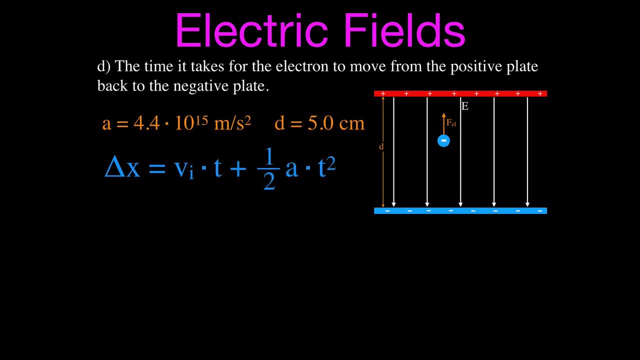 And let's see, We're going to have the time. The time we're going to use are kinematic equations And that says that the distance- OK, delta x, delta y, the change in the distance, the change in position, is equal to the initial velocity times the time plus 1 half a. 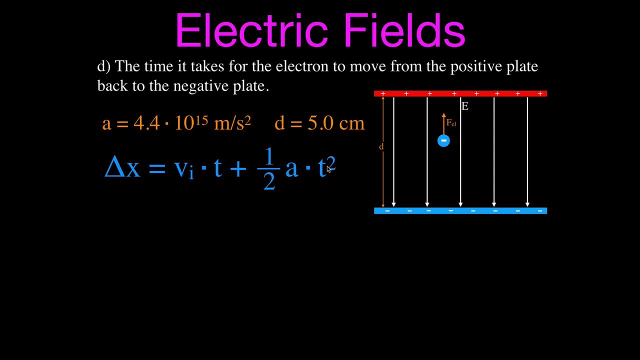 the acceleration times, the time squared. Now we're going to assume, when we have the particle here, that it did not have any initial velocity. So that means this initial velocity is 0.. And initial velocity is 0 times t is also 0.. 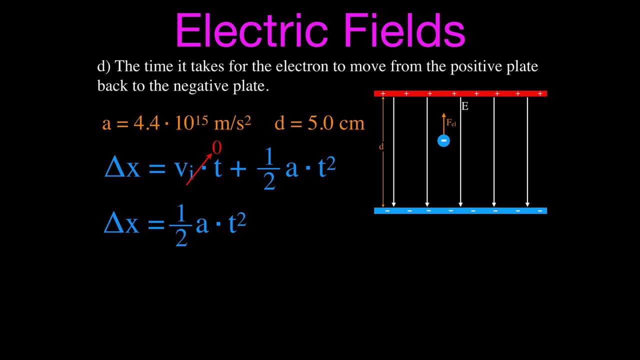 So our equation reduces to delta: x equals 1, half a t squared. And we want to know the time. So we're going to do the same kind of thing we did, basically, when we solved for the velocity in the kinetic energy: We're going to multiply by 2, divide by a. take the square root. 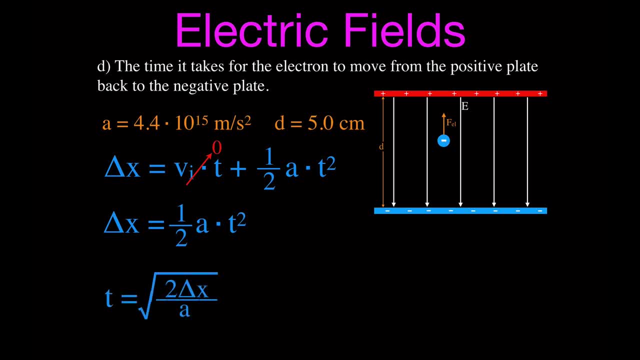 And we get the time is equal to the square root of 2ax, the distance which it's moved divided by the acceleration. Plug those values in And you get that the time it would take would be 4.77 times 10 to the minus 9 seconds.